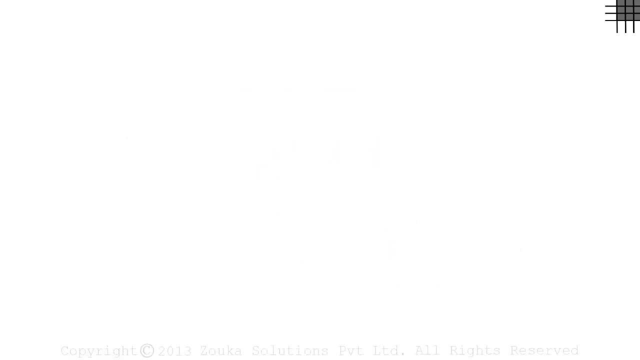 Let's understand the various categories of numbers that come under real numbers. Real numbers can broadly be classified into rational numbers and irrational numbers. Irrational numbers are numbers like root 2, root 3, pi, etc. These numbers cannot be expressed in a fraction form. 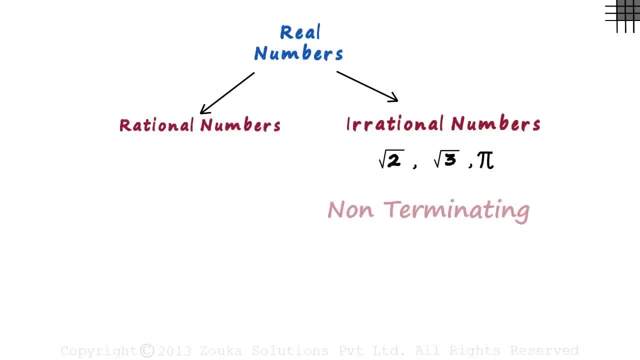 Like p divided by q. They are also called non-terminating, non-recurring decimal numbers. And rational numbers are broadly classified into two types. Fractions are in the form p by q. Fractions are sometimes referred to as non-integers. 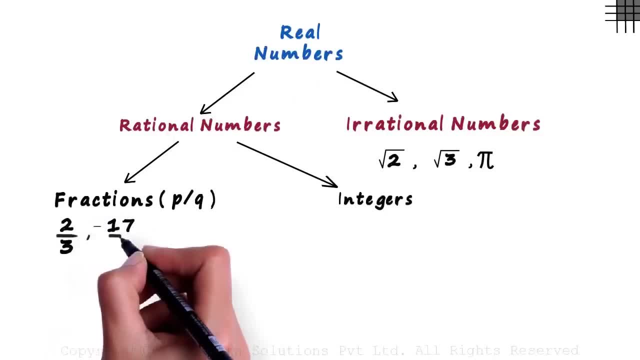 They are numbers like 2 by 3 or minus 17 by 12. The numerator and the denominator have to be integers. p and q cannot be anything like root, 2 or pi. Integers are basically fractions with denominator as one. They are also broadly divided into two categories. 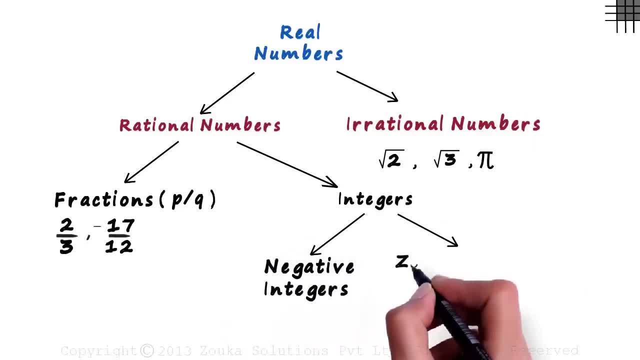 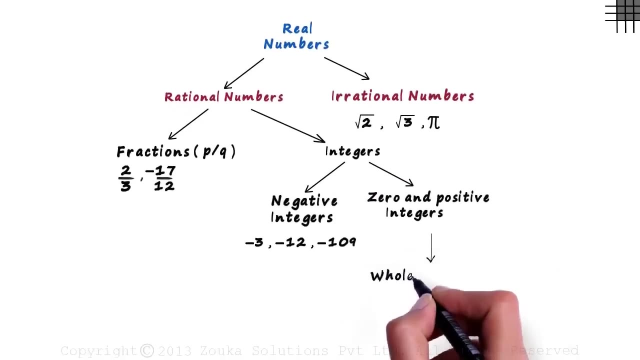 Negative integers and the second category is zero and positive integers. Negative integers are like minus 3, minus 12,, minus 109, etc. Zero and positive integers are called whole numbers, which start off with zero and go on to infinity. So whole numbers include all positive integers along with zero. 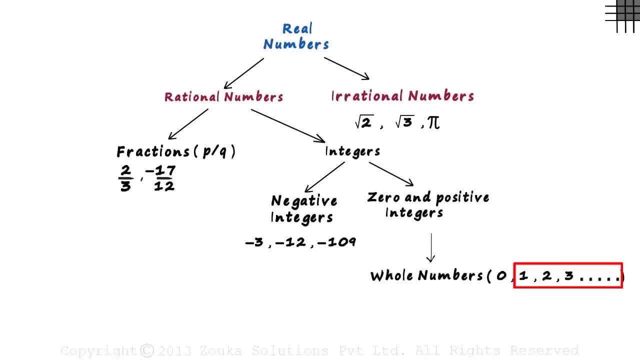 And these positive integers also have a special name. They are called natural numbers, which include all positive integers starting from one. So real numbers pretty much include all the numbers you've seen, All numbers which can be expressed as p by q, which are rational numbers. 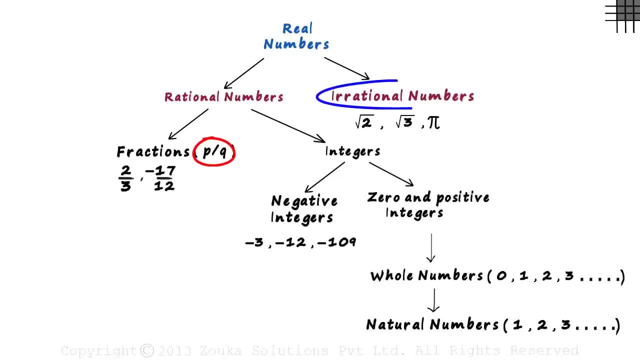 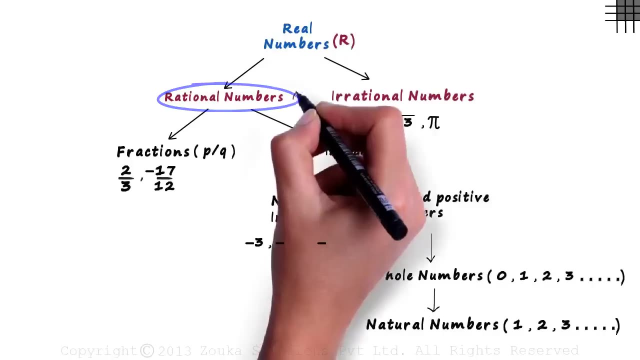 And also the ones which cannot be expressed as p by q, called irrational numbers. All the categories you see are given one-lettered names. Real numbers are called r, But not all categories are named based on the first letter. Rational numbers are called q and irrational numbers are called p or q-. 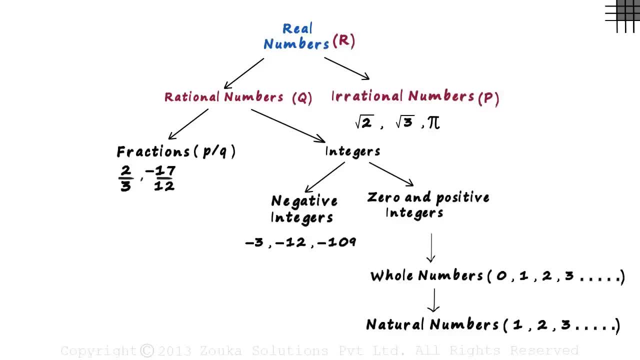 The entire set of numbers is given the letter: So p is an entire set of irrational numbers. q is an entire set of rational numbers. So p is an entire set of irrational numbers. So p is an entire set of rational numbers. Set of integers is called i or z.